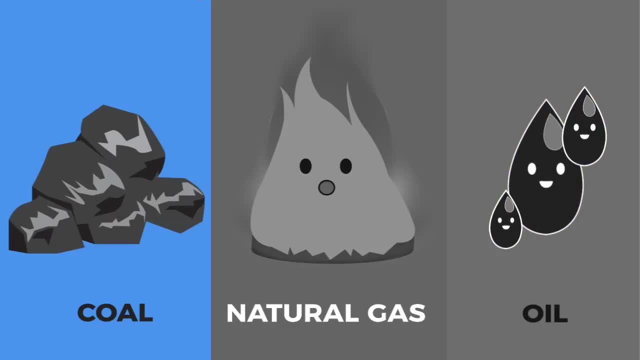 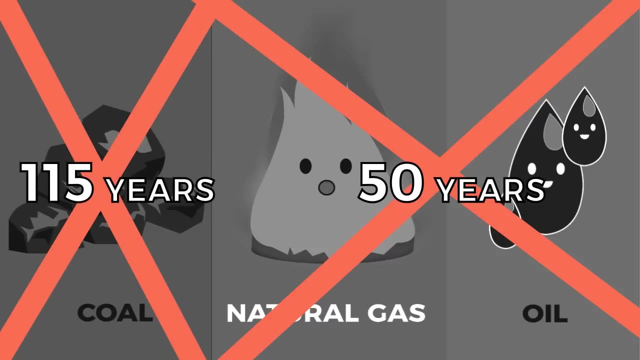 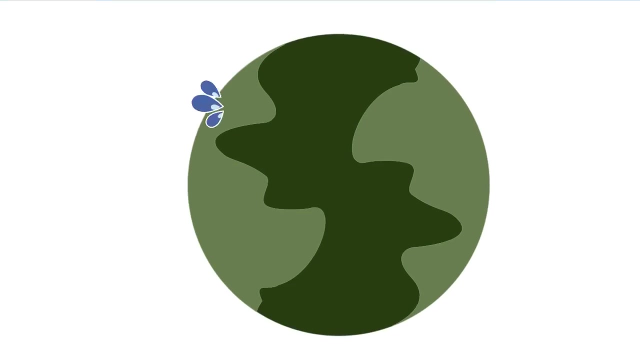 zenie, we may run out of oil and gas in the next 50 or so years and coal in the next 115 years. Not only are these non-renewable resources going to run out, they are also polluting our planet and contributing to climate change. The sun's energy, on the other hand, will 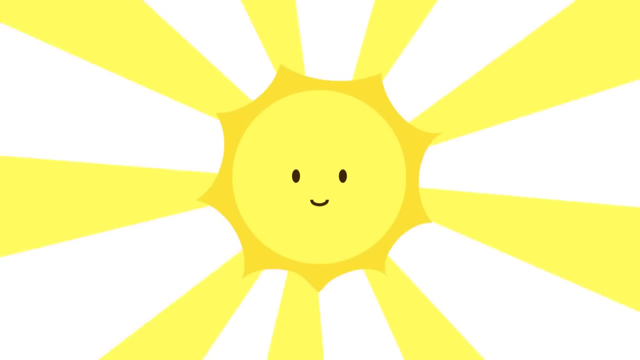 not run out for the next 5 billion years. That makes it a renewable resource. Other renewable resources like wind and water can also provide us with energy, But even all the energy we can get from all these sources added together is still less than 1% of the 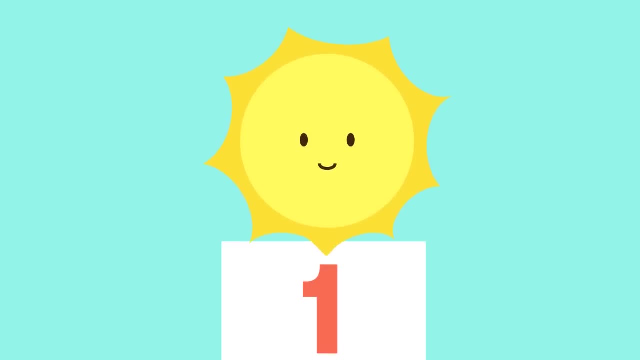 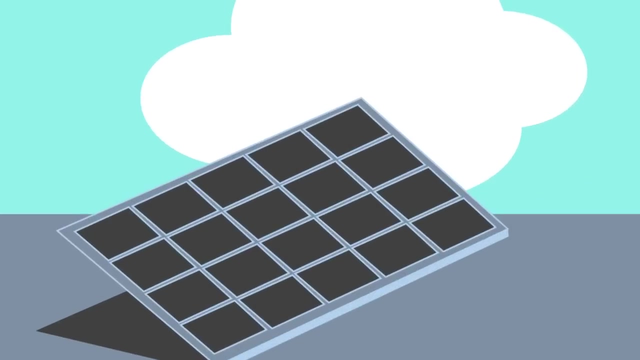 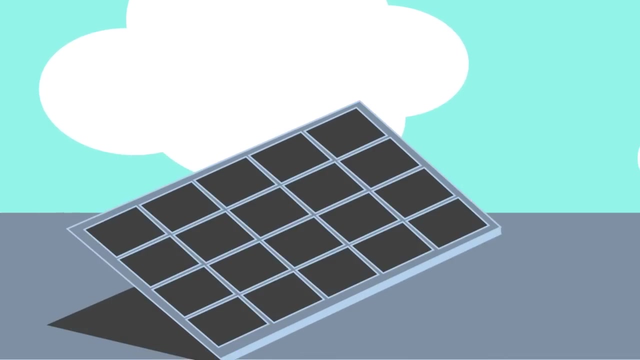 solar energy reaching the Earth. It's clear that the potential of solar energy massively outshines its competitors. How exactly do we harness solar energy? Solar panels directly convert sunlight into usable electricity using special materials like silicon. Another way to harness solar energy is through a process. 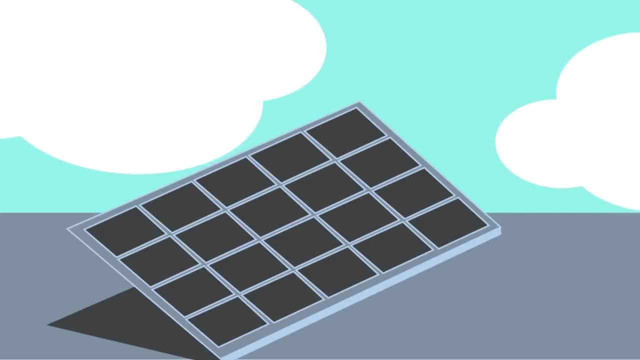 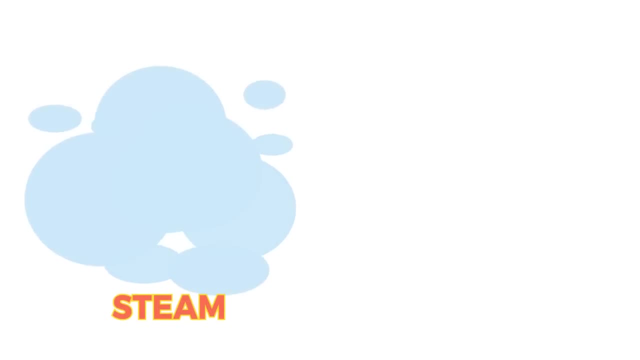 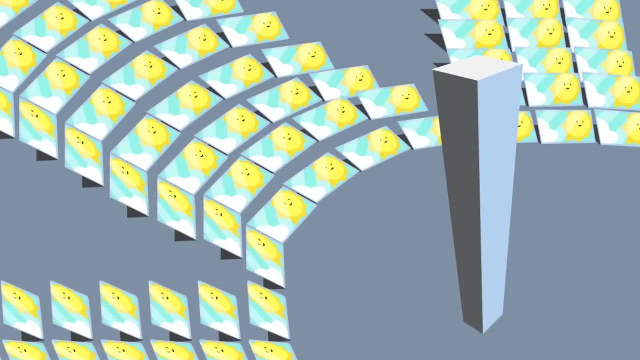 called concentrated solar power, which uses thousands of mirrors to reflect sunlight onto a tower. The heat captured in the tower makes steam that flows through a steam turbine, which generates electricity. But even though we have these promising technologies to capture solar energy, there are still many challenges with using solar energy. 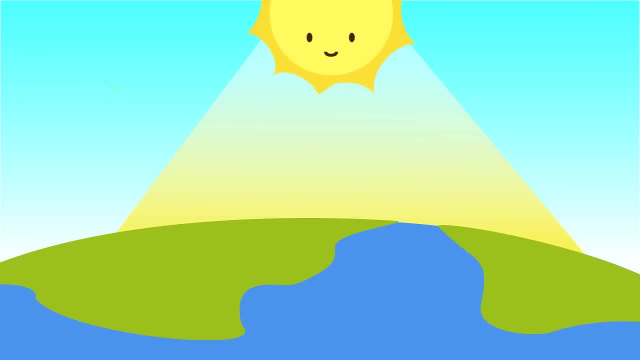 on a large scale. For example, the amount of solar energy we can harness can change based on place and time. Some parts of the world get much more sun than others. Solar panels in the Sahara Desert will produce more energy than those in Seattle, But even in 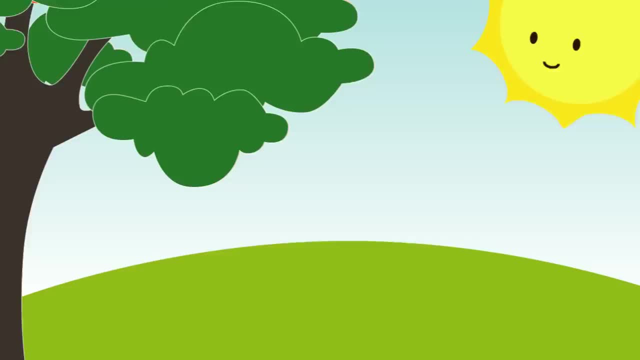 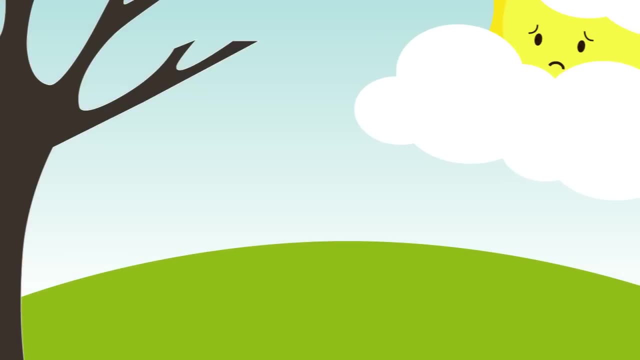 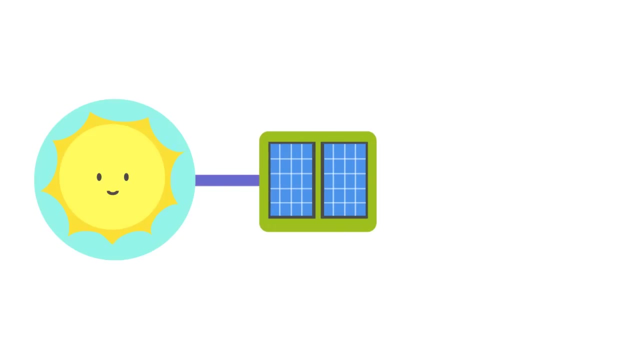 the sunniest places, the sunlight still isn't constant. The changing of seasons, the cycle from day to night and even clouds in the sky can reduce the amount of available energy. This is the reason why solar panels are so important: To make solar energy usable when and where it's less available. we need to improve energy. 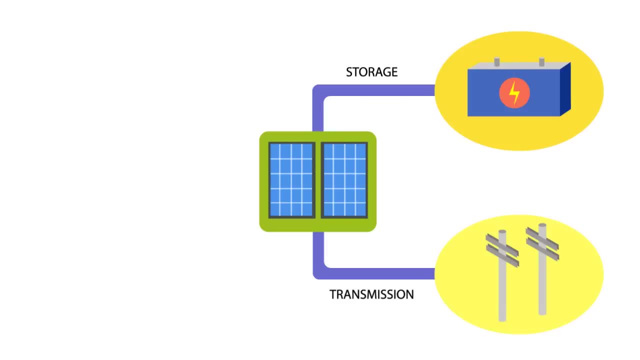 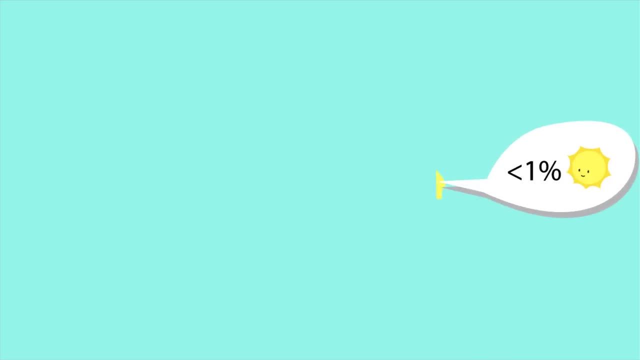 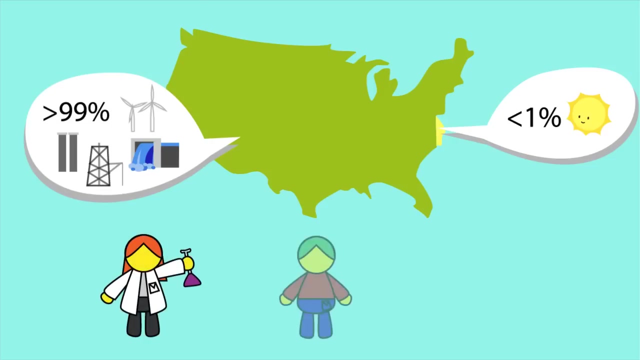 storage and transmission systems. Above all, we also need to make solar technologies more efficient and less expensive. Currently, less than 1% of all energy produced and used in the United States comes from solar energy, But as more researchers, private citizens,